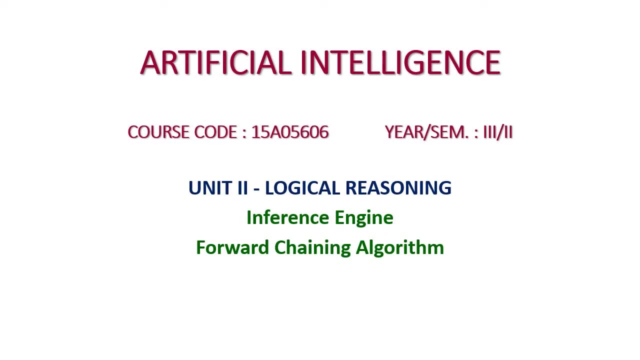 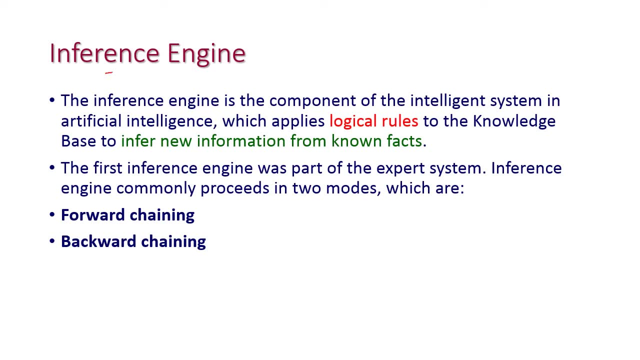 algorithm in detail and in the next video we will see the backward chaining algorithm. First let us see what is inference engine. Inference engine is the component of intelligent system in which the logical rules are applied to the knowledge base, to the knowledge base. Knowledge base means kb, and why: to infer new information from known facts. to infer new. 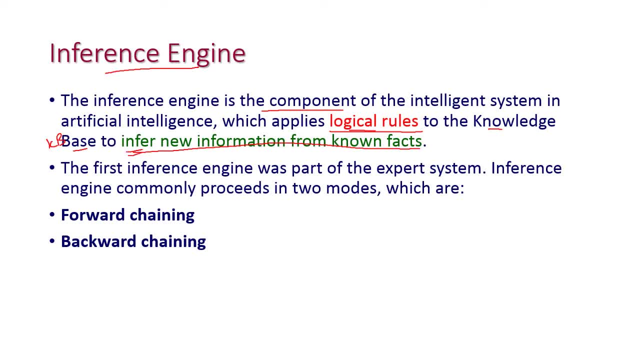 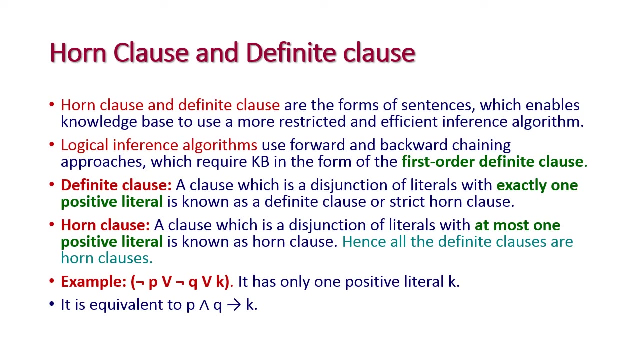 information, that is, we are going to extract new information from the already existing information Which are stored in knowledge base. The first inference engine was part of the export system and here there are two modes. first one is forward chaining and second one is backward chaining. The important classes in inference engine are horn class and definite class and 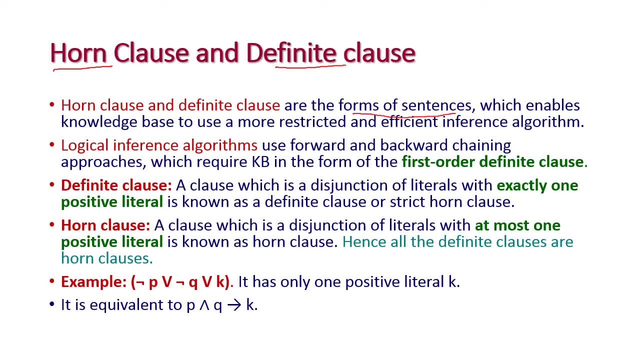 these two are different forms of sentences, simply, which are available in the knowledge base. And what is the purpose of these two classes means to improve the efficiency of inference algorithm, and here the logical inference algorithm uses the forward and backward chaining algorithms, and that required the knowledge base and the information in the knowledge. 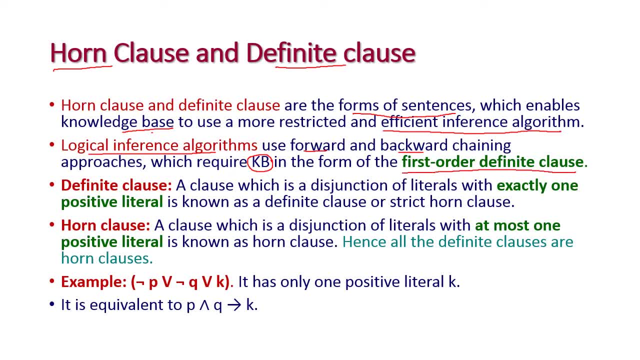 base should be in the form of first order definite class. and let us see what is definite class. It is a class which is a disjunction of Littles, which is a disjunction of Littles with exactly one positive literal, is known as definite class, or it is otherwise called as strict. 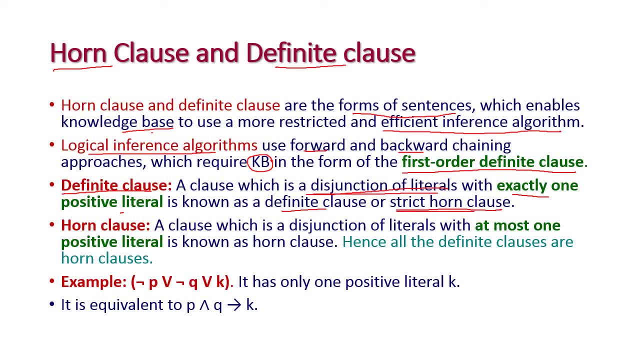 horn class and second one is horn class. It is a class which is a disjunction of litterals with at most one positive literal, with at most one positive litter with at most one positive liter Of positive literals. is called as horn class, hence Hall definite classes are: 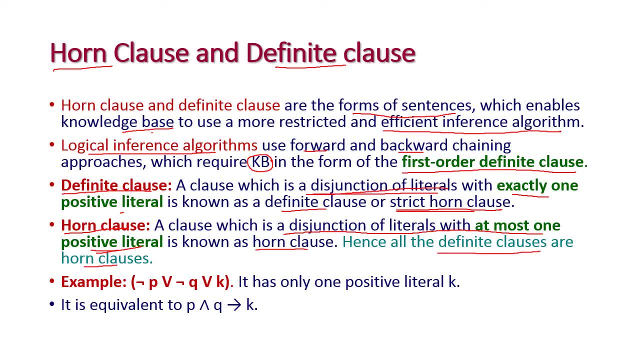 horn classes. let us see one example for this. so in this example we are having: this is negative literal and this is positive negative literal and K is positive little and the symbol, the symbol is disjunction symbol. so we are having disjunction of disjunction class. this class is called as disjunction class. 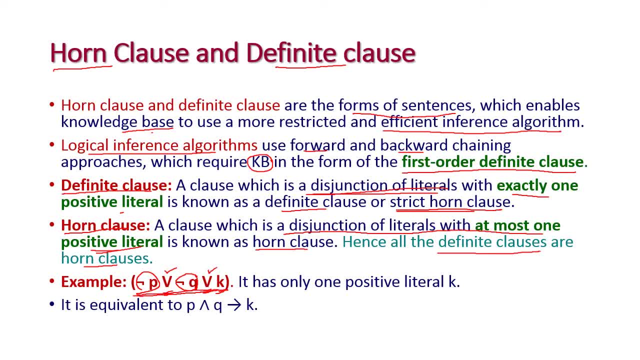 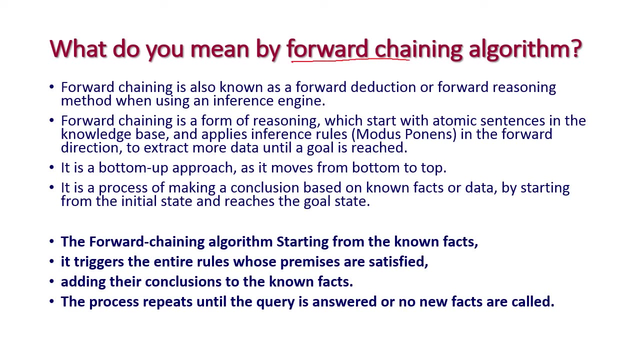 because we are using only the disjunction symbol and we are having only one positive literal. hence this is called as which class, horn class and definite class. the next question is: what do you mean by forward-chaining algorithm? this is one of the important concept in this second. 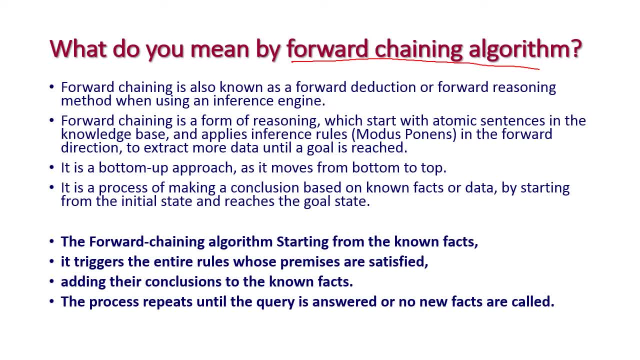 unit. the forward-chaining is known as forward deduction or forward reasoning method when using an inference engine, and forward chaining is a form of reasoning which starts with atomic sentences in the knowledge base and applies inference rules. that is modus ponens in forward-chaining algorithm. 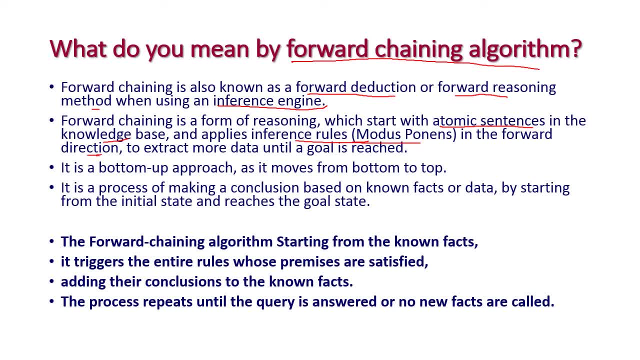 direction to extract more data until goal is reached, and it is a bottom up approach that means it moves from bottom to top. It is a process of making conclusion based on facts or data, by starting from initial state and reach the goal state, And the forward chaining means the forward chaining algorithm starts from known facts. 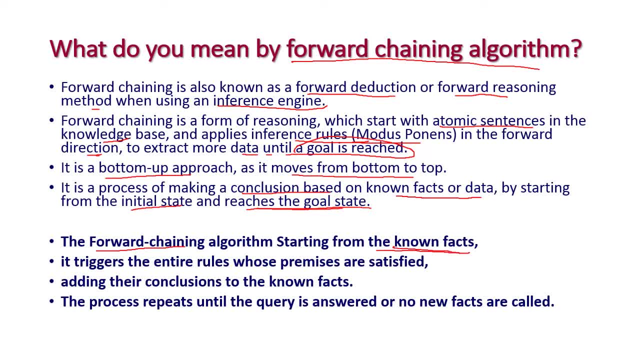 Known facts are available in the knowledge base and triggers the entire rules whose premises are satisfied, adding their conclusions to the known facts, And this process repeats until the query is answered. Until the query is answered. Until the query is answered, This is called as forward chaining algorithm. 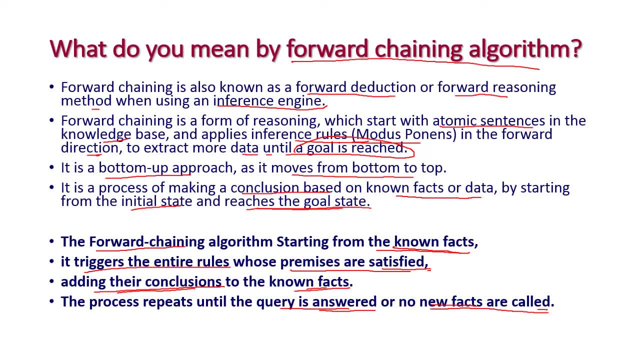 Here there are no new facts which are called, So this is called as forward chaining. So this is called as forward chaining. Forward chaining means the starts from known facts and it triggers the entire rules in the knowledge base whose premises are satisfied and adding their conclusions to the known. 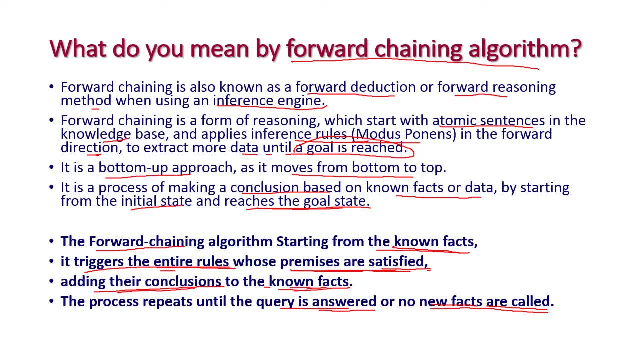 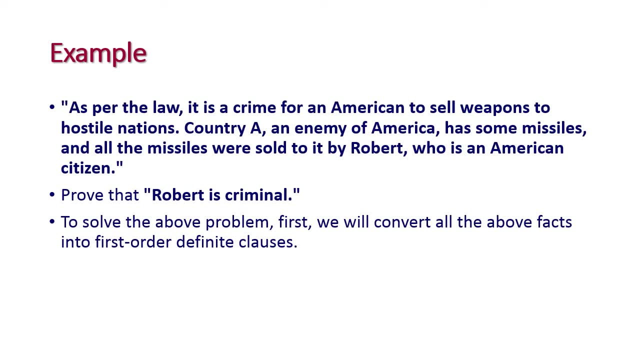 facts And this process, these three processes will be repeated until the query is answered or no new facts are called. this is called as forward chaining algorithm, as forward signing. and now let us see one example here. they will give you a set of statements. the given statements are: as per the law, it is crime for an american to sell weapons to hostile. 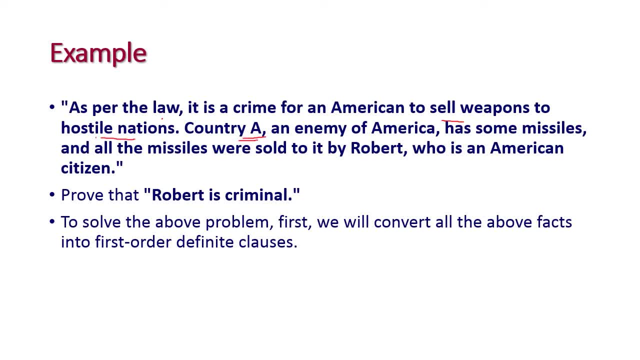 nation, a country, a, an enemy of america, has some missiles and all missiles were sold to it by robert, who is an american citizen. so from these statements we need to prove that robert is a criminal. to solve the above problem, first we have to convert all the above facts into first order. 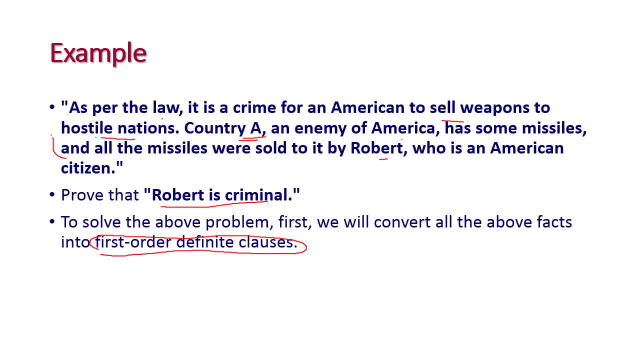 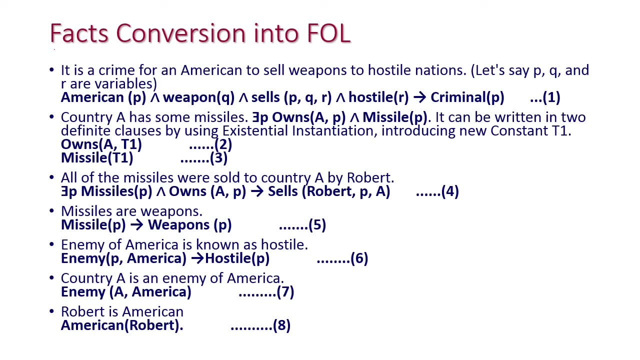 definite classes and this is very important. first, we need to convert all the given english statements into first order logic statements. the facts, conversion into first order logic, that is, the given english statements will be converted into first order logic form. it is crime for an american to sell weapons to hostile nations. 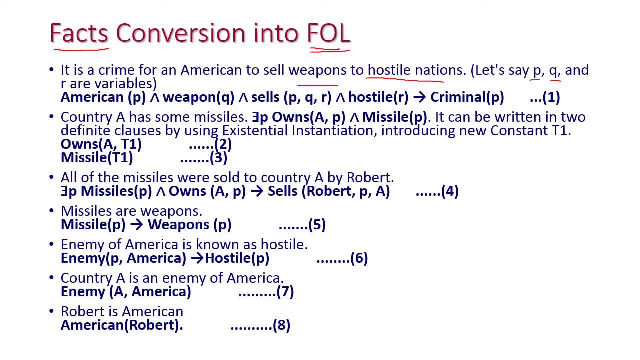 here we are having three different variables and we are going to apply these variables in american weapon and hostile nation, that is american of t conjunction, that is, and weapon of q and sells p, comma, q, comma r, that is p sells q to r, and hostile of r. 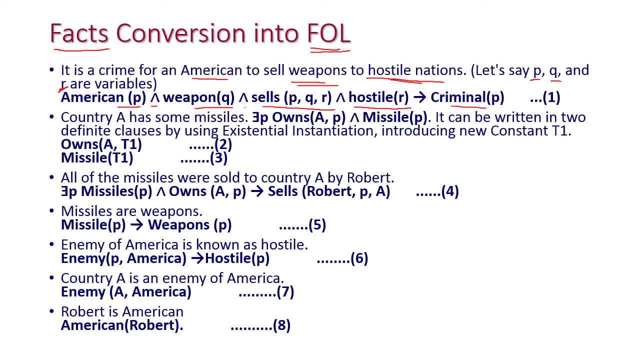 implies criminal of p. this is the first statement. first statement will be converted into first order logic form. and the country a has some missiles. the country a has some missiles. some missiles means existential instantiation, isn't it? so there exist p owns a comma, p and missile of. 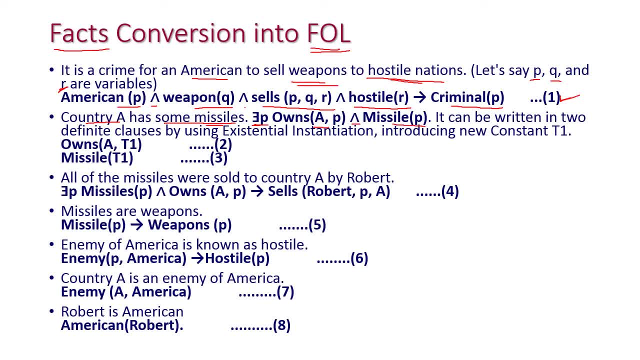 p, a comma p and missile of p. it can be written into definite class by using existential instantiation. and for to replacing these thing, we are going to introduce another variable: t one hence owns a comma t. one is the second sentence and missile of t is the third statement. 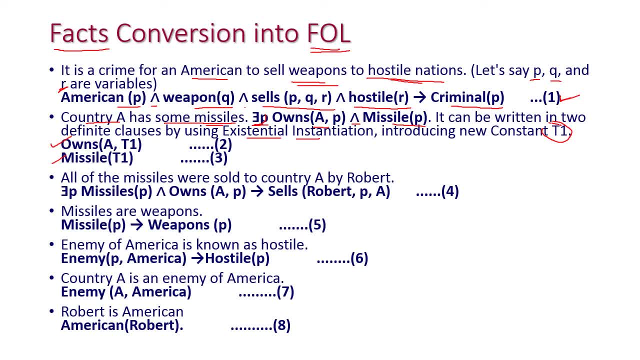 And next one: all the missiles were sold to the country A by Robert. There exist P, missile of P. There are some missiles owns A P, Owns A P. that implies sells Robert P A. So this is the third statement. 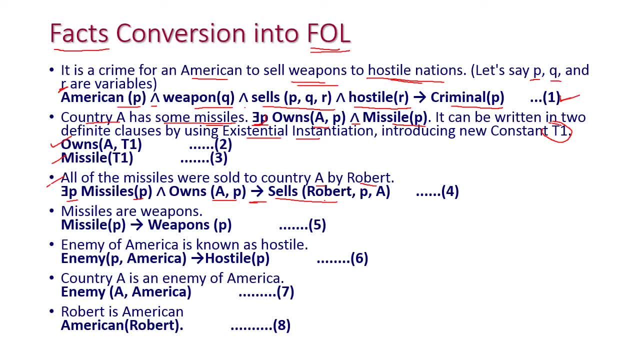 And next statement is: missiles are weapons. Missiles are weapons means missile of P implies weapons of P. And this is the fifth one. And next statement is: enemy of America is known as hostile, Enemy of P. America implies hostile. And next one country, A, is an enemy of America. That is enemy of A. 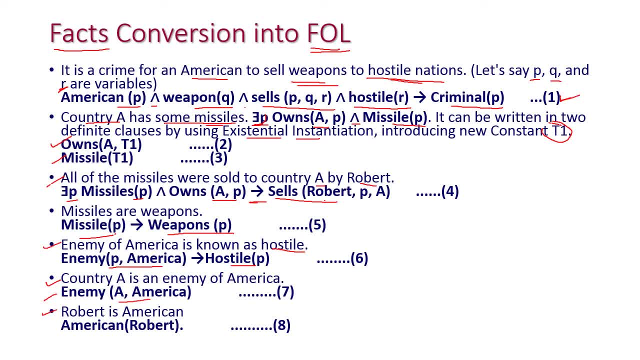 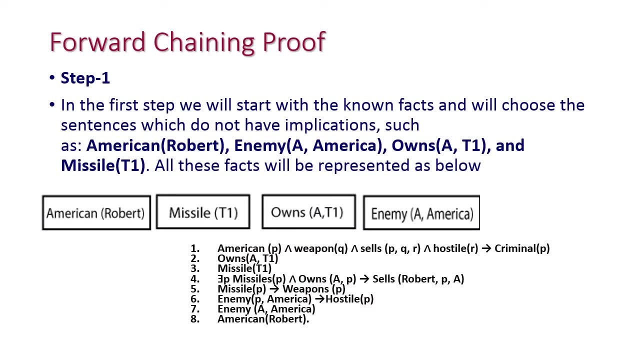 America. And the last one is: Robert is American, American of Robert. So this is how we need to convert all the facts, that is, English statements, into first order logic statements. And now let us start the forward chaining proof, First step. In the first step, we will start the known facts. We will start only from the known facts. 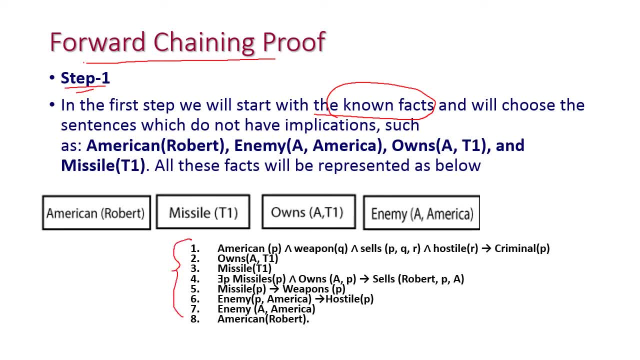 And then we will choose from the sentences. Here I gave all the sentences which do not have implications, which do not have implications. So we will choose the sentences which do not have further implications. First, one is American of Robert. We will take that sentence first And enemy A America. And third, one owns A T And the last one is missile of T. 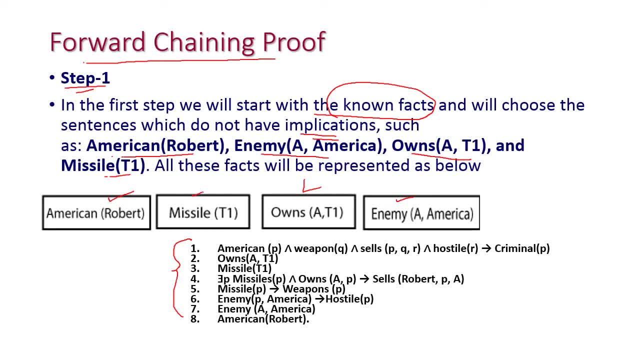 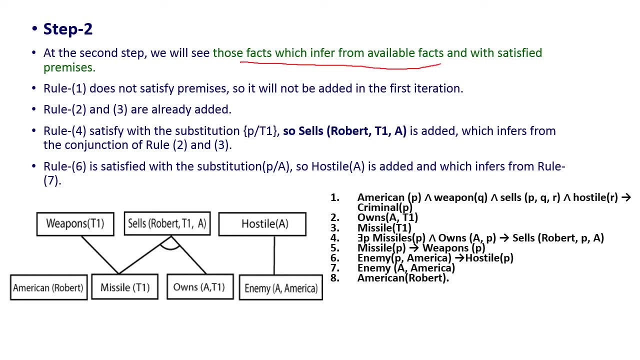 So all the sentences here, only so, second, one, third, one enemy of a and American Robert. in the second step we will see the facts which infer from available facts, the facts which will infer from available facts that to be satisfied the premises, and let us see. 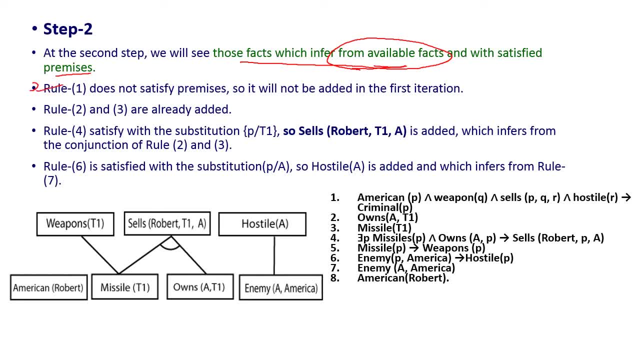 all the rules one by one. first we will take the first rule which. that does not satisfy the premises, so we will not add this one first rule in the first iteration and the rule 2 and rule 3 are already added. rule 2 is here, rule 3 is. 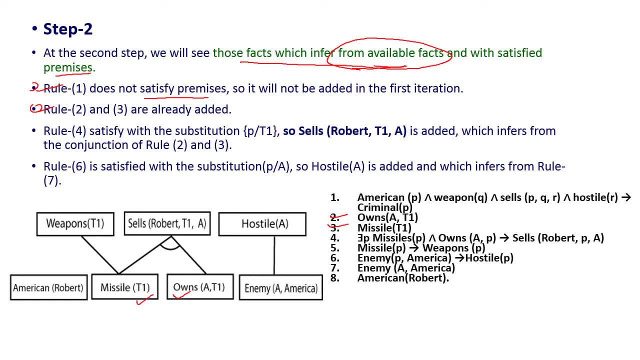 here and those two rules are already added and rule 4, which is satisfy the substitution t1 in the place of P. so cells robot comma t1 comma a is added. cells robot comma t1 comma a is added, and that will come. the conjunction of rule 2 and 3. conjunction means so this: 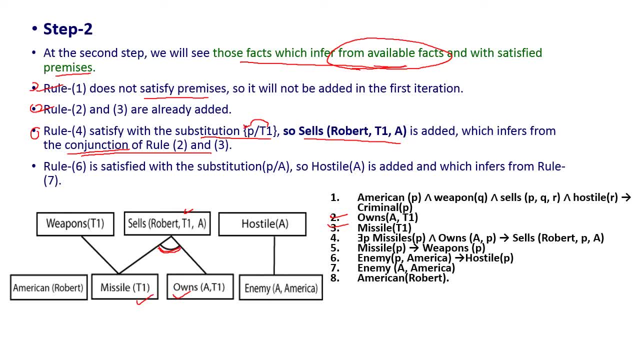 is the conjunction rule. if we do the conjunction of rule 2 and rule 3, then we will get this rule 4. so rule 4 is added here and rule 6, which is, satisfies the substitution of a in the place of P- so was I love a- is added, which infers a. 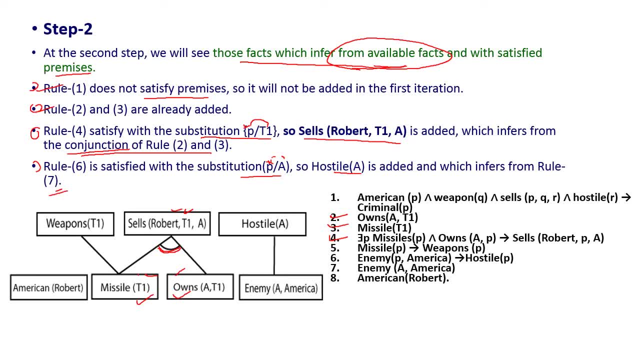 from rule 7. rule 7 is here. rule 7 is here and this a will be replaced in the place of P. then we will get wholesale of P. that is taken from rule 6. okay, so from here this will be added, that is, rule 7 will be added here in step 3. we will. 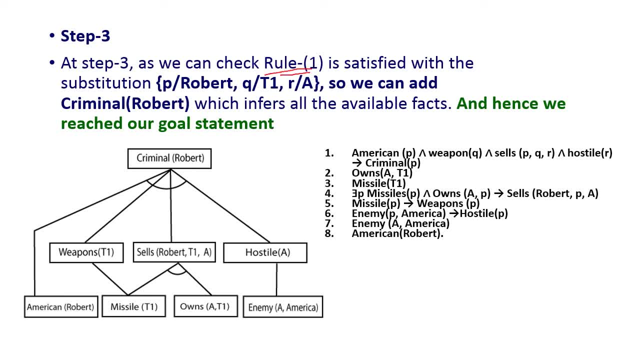 check rule 1, which will be satisfied with the substitution of robot in the place of P and t1 in the place of Q, a in the place of R and Robert. here we can include Robert. see this: Robert will be included here and t1 will be substituted in the.